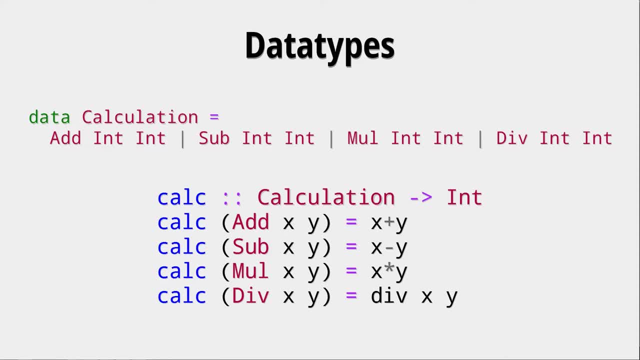 So now the question might be: how do we work with our own data type? Well, it could work like this: You can use your constructors in a pattern matching, just like you did with lists, Because, think about it, a list has a list. You add two constructors- The prepend or colon constructor, or whatever you want to call it, and the empty list. 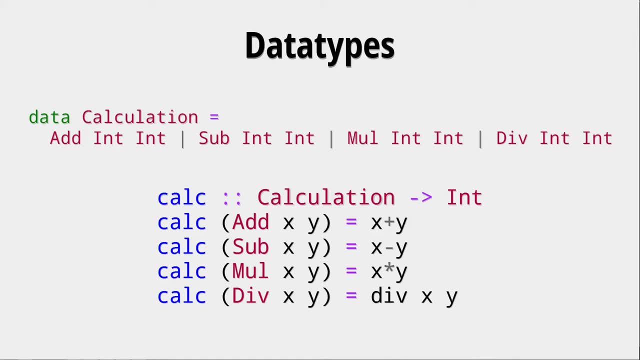 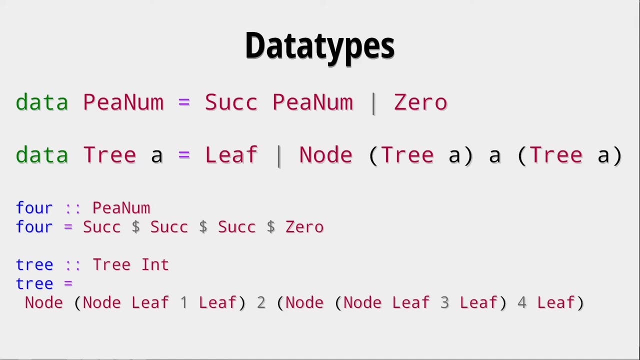 And you use those in the pattern matching. Now here we have other constructors like add, sub, mull and diff, and now we can use them like that here. Okay, so let's look at recursive data types. Here we have a new one, the tree of A, and this is a special kind of data type. 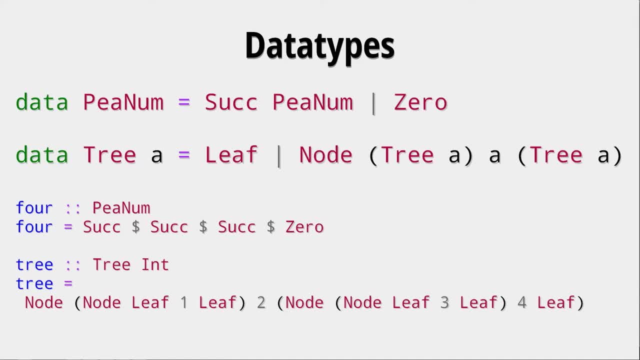 Because it now has a polymorphic type in it. So this is not just any tree, At least not in the tree that we see down here. This is a tree int or an int tree or whatever you want to call it. It is defined as either a leaf or a node that has some value in 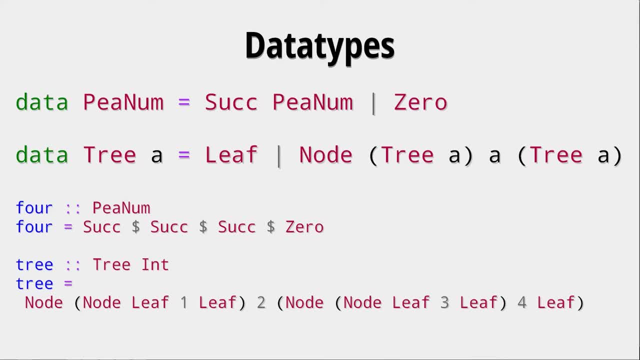 its middle and then a left and right subtree. It's very important to have this A here, since of course we don't want our tree to have different types on different levels. That would be weird and it wouldn't work because there would be no type safety. But here we see how some of 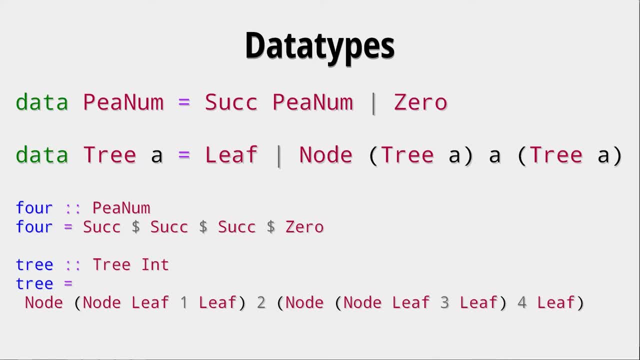 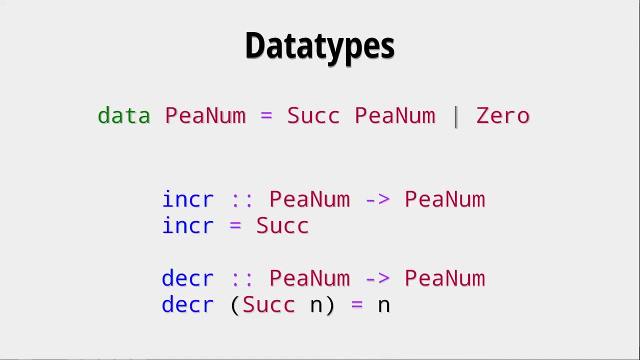 those types can be constructed. We also see that this dollar sign can be used in a constructor. You can basically treat a constructor just like a function, and here we see an example of a tree tree. okay, so how do you work with those data types within your functions? well, it's actually. 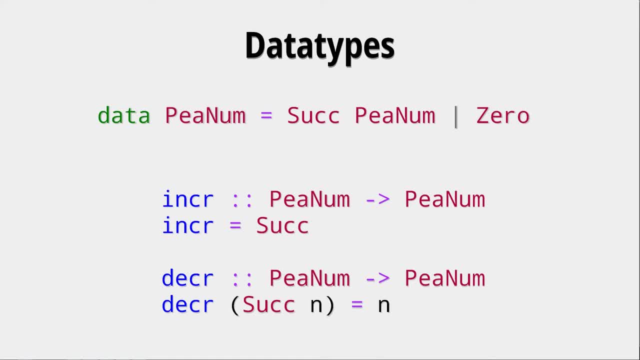 rather easy. so here we want to have an incur function, so an incrementation function. and on this sort of number definition, this is very easy. you just put a successor in front of what number you have, and here we see something very interesting. we use this successor constructor.